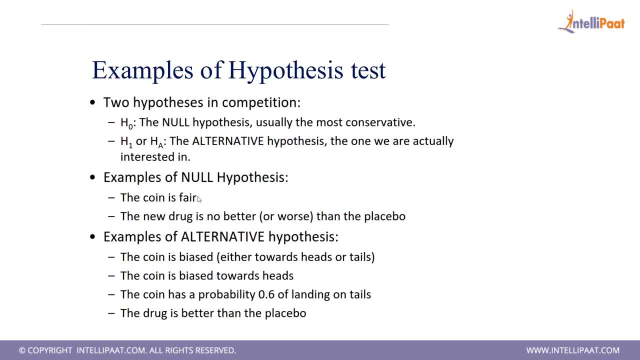 claim that the coin is fair. Right, This is your null hypothesis saying that the coin is fair. Alternate: you say that coin is biased. It is not either biased toward heads or tails, so that you're the coin claim was saying that the claim was: coin is fair and we are tossing. 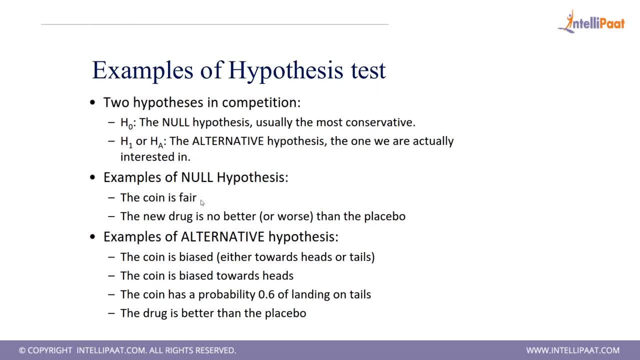 it something right and the null hypothesis supports the claim and alternate hypothesis doesn't support the claim. That is what you can. you can look for as null hypothesis and alternate hypothesis. Okay, One one else. Another example is new. a drug has been come and they want to do some test. 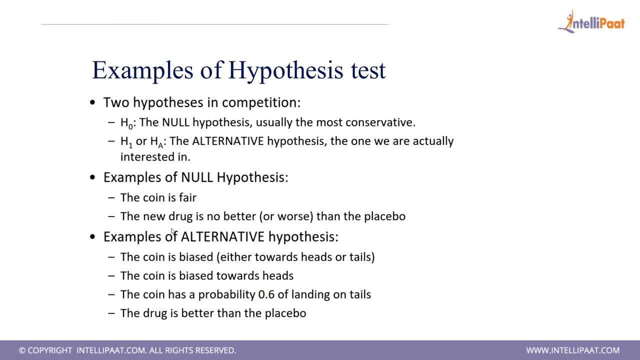 and all. So alternate, null hypothesis: that new drug is not better than the earlier placebo or something. So it alternate hypothesis: it supports that the drug is better than the placebo. Those things are there when, when you look for the claims, You will have null and alternate hypothesis. Each are one is supporting, one is disclaiming. 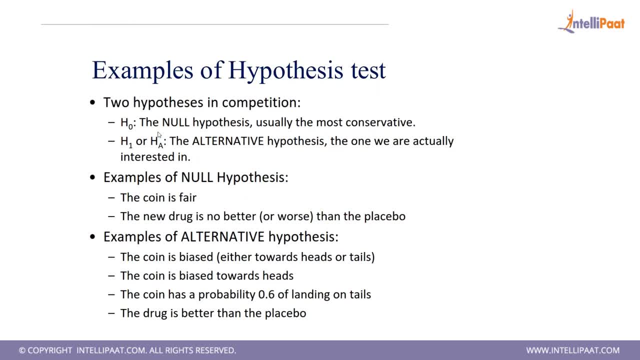 the claims, whatever you need Right. So we need to test which which comes in to be true. So that is where a given claim is being said: you're one is one guy to two people are there, which is supporting to you and which is not supporting to you. Those things you can consider. 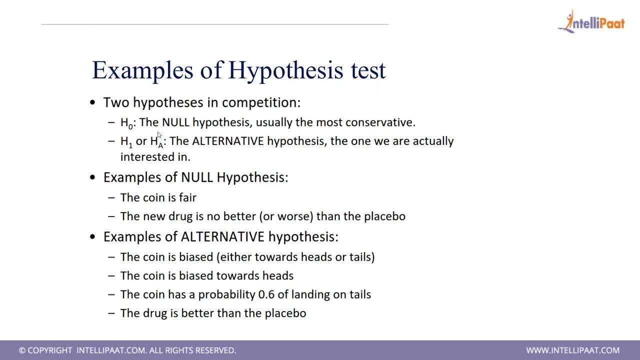 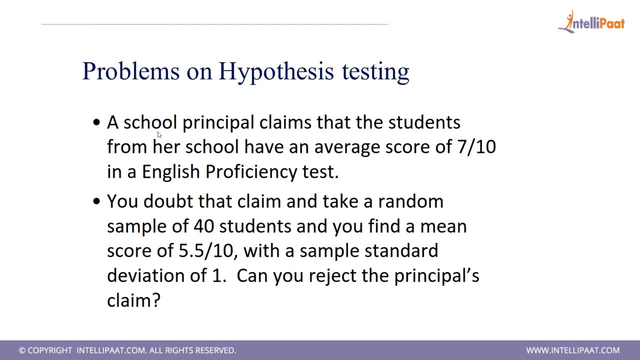 as non alternative hypothesis. You have made a claim And one is supporting you, one is not supporting you. is what alternate and null hypothesis is right? yeah, problems on hypothesis testing is a school principal claims that the students from her school have an average score of this one seven out of ten, probably like seventy percent in english proficiency test. 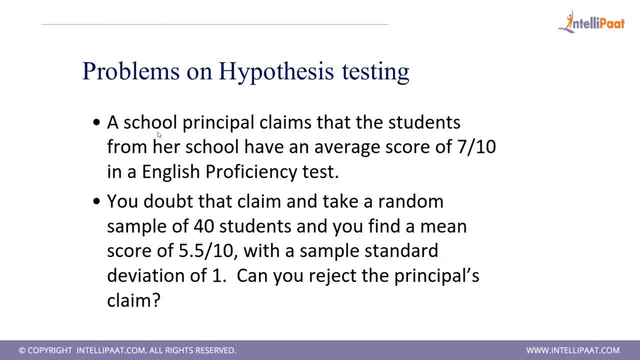 whatever score comes in, seven out of ten bands, those things are there. so she claimed it. right now, as a statistician, what do you want to do? you need to cross check that if it is true or not. so how you do that? you take a sample of a of a class, say you. you take a random sample of 40 student. 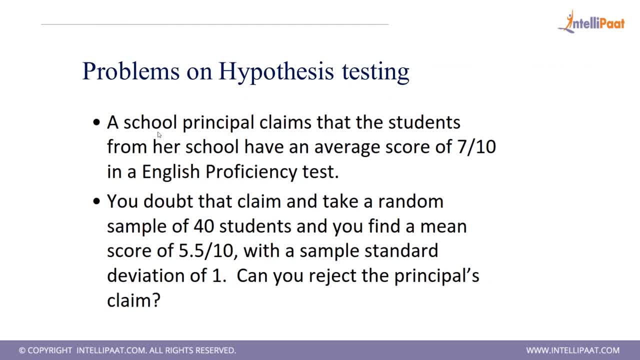 and you find a mean score of for them, the entire 40 student. you find you found out that 5.5, 5 is the mean. uh, where average every student you are getting out of 40 students, 5.5 is your mean right and the standard deviation is one. if you calculate, if it will give you a. 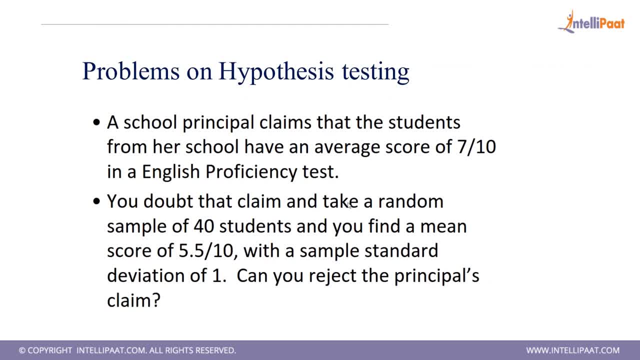 uh vector of 40 students. you feed in and you get um. probably the mean comes in to be 5.5 and standard division is given. can you reject the principal's claim? either this data supports the claim or rejects the uh, or no, doesn't support the claim, right. 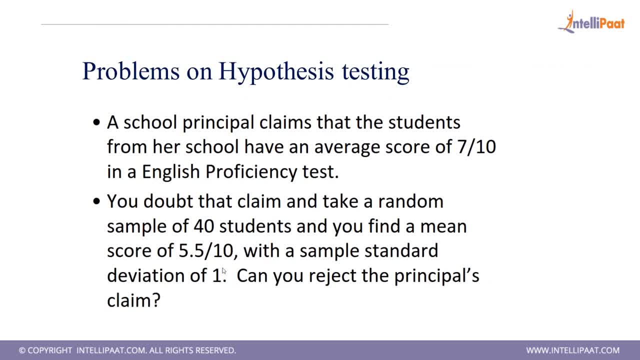 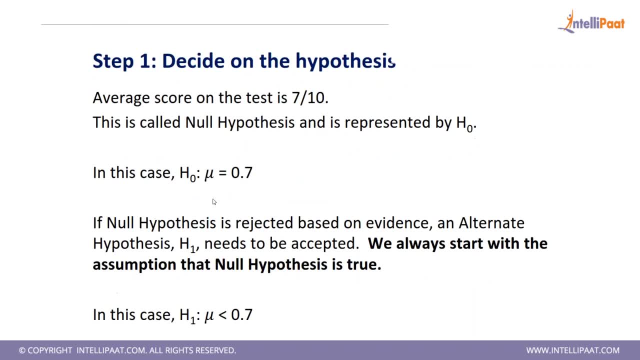 okay, that is what you're trying to do it here. okay, first thing is, what we need to do is we need to try it. we need to frame the hypothesis. what actually null hypothesis is, what actually, uh, ultimate hypothesis one is supporting, saying that, yes, you get uh, 70 percent, seven bands out of ten. 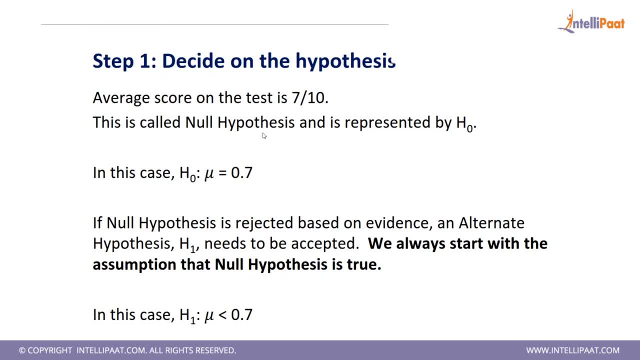 uh, as per the principal's claim, is your null, null hypothesis. one is no. you don't get seven bands. is your alternate hypothesis right? those things are way, or you probably get lesser than that. so that is where your alternate hypothesis is your. you're not accepting the claim made by principle. 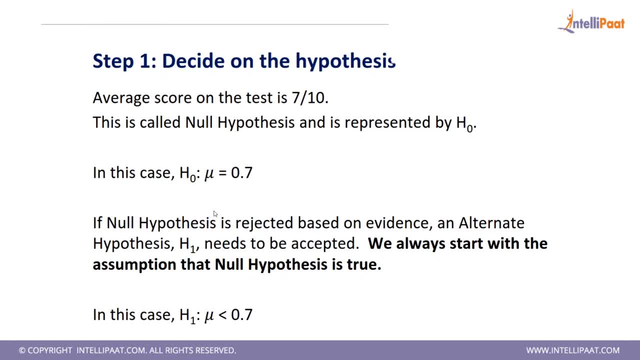 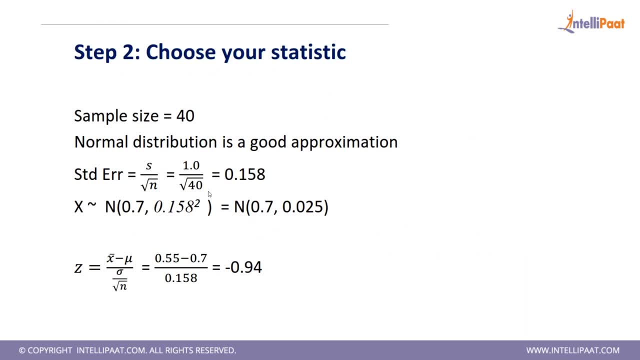 right, these are the first step. you set your null and alternate hypothesis. then you take the statistics here saying that the sample size you took, it's 40- and you try to calculate the standard error. so what would be the standard error formula? for that is standard deviation to that of number of elements or sample size. 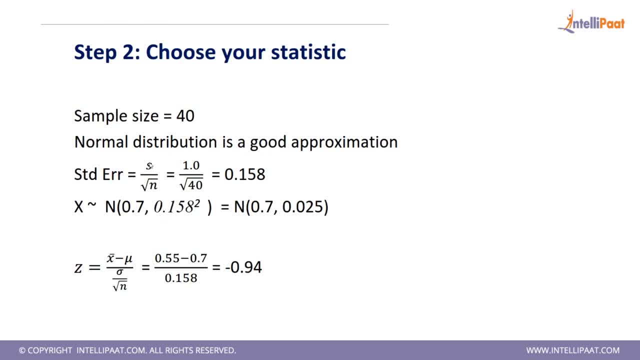 right sample size: standard deviation to that of unless root of the number of elements involved in it. that gives you the standard error. and if you check the z-score, so what? what you're? you're doing this, you're passing this coming here is five. five when you take the sample. okay. 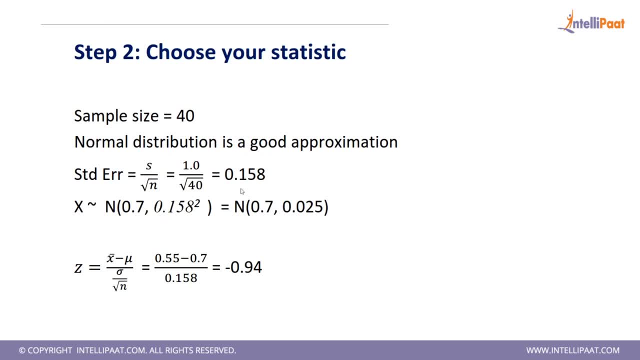 you. so this standard error would be passing here. right, this would be passed. X is your, the value of which you got from the sample of 40 student five point five week. you brought it and your seven bands were there divided by ten. so you're, you're. 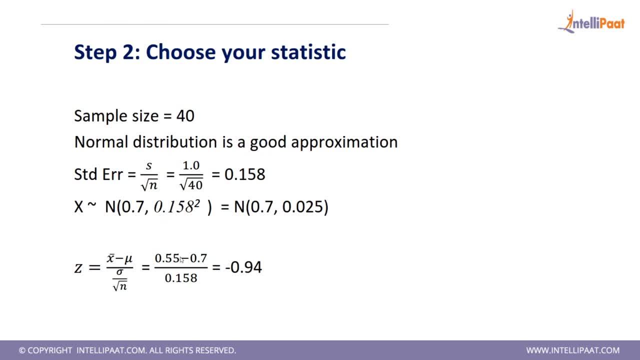 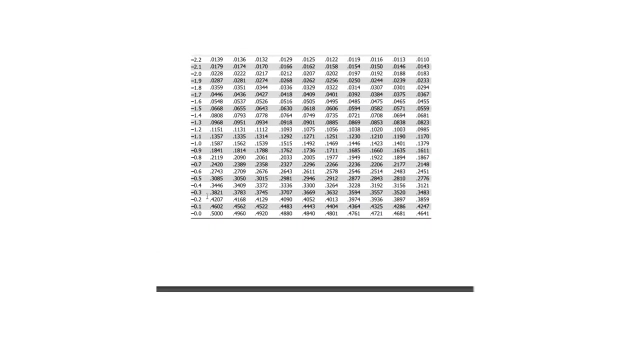 getting point seven, year five, point five by ten ten, you get point five, five, right, whatever the value company. so you you got the negative value here. if you check the value disease in the z-score table, minus 0.94. if you go here, minus 0.99 and 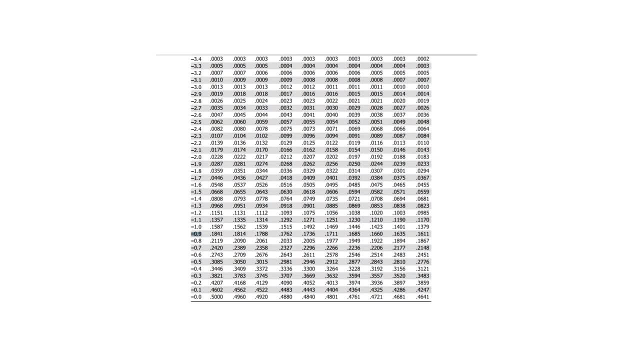 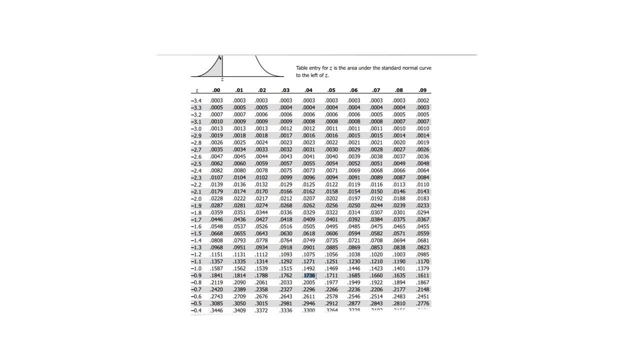 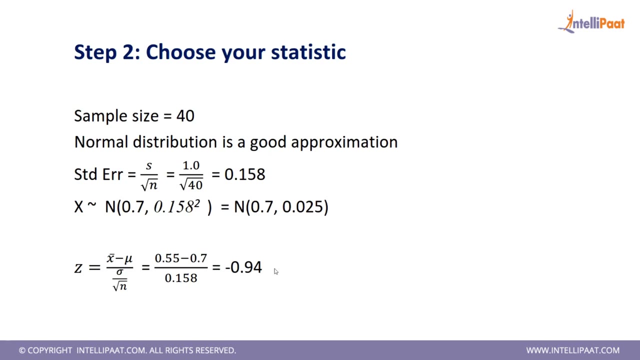 4 right 17%. you get 17.36. okay, one thing is you got some support or something, did not you? you got it before that. you need to consider what significant level you are looking for. either you are looking for the entire data to be in 95%. 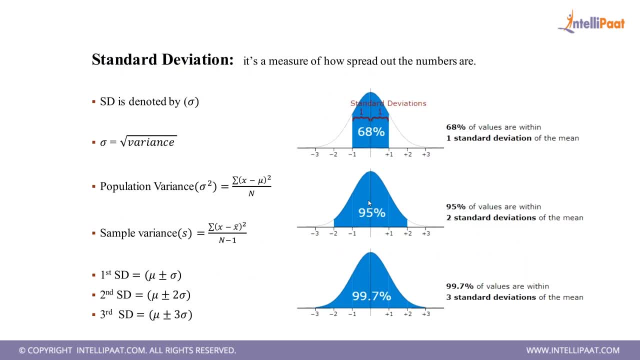 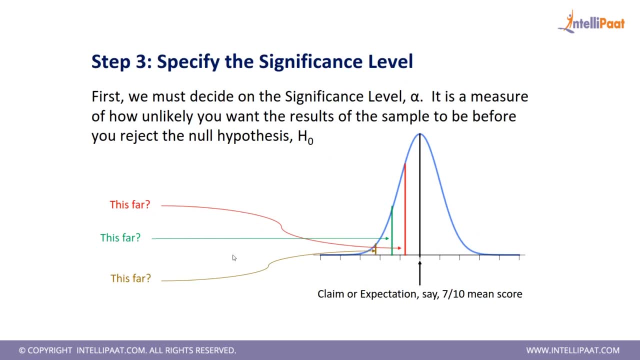 range. the claim should be the range of 99 percent sure or 99% sure. for that you are setting the significance level. so this is what: first standard deviation, second standard deviation or third, standard division, how far you are looking for the claim to be. so if you do at first. 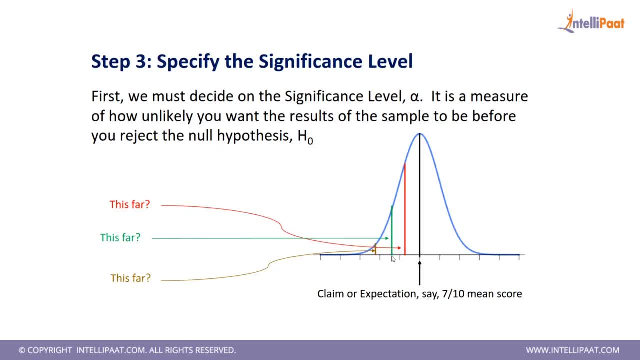 standard deviation it will look for 60. so mean would be somewhere around 50% here. so the value will be pointing somewhere 17% here. you consider the entire population, so mean would be 50% here, 50% here data and your value which we got is 17%, which is somewhere here earlier, the entire. 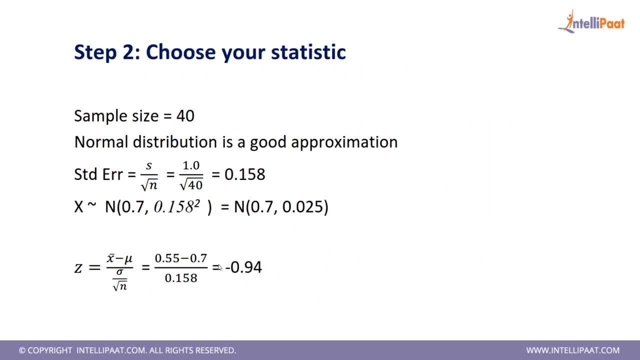 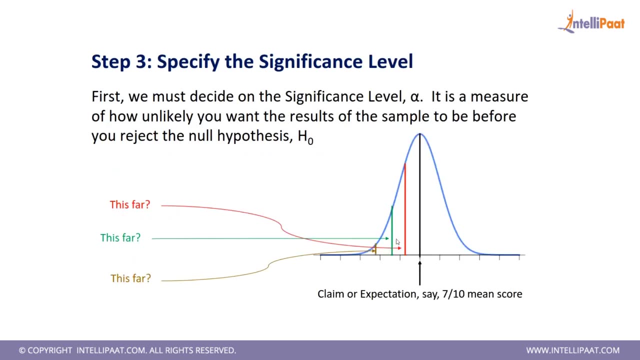 population used to be point seven. okay, but as per the claim, point seven. but you, when I take the sample out of it, right, when I take the sample out of it, it is the. the mean value is coming somewhere here. the probability is coming somewhere here and at this point I'm just checking if it is 95% significant or I'm just 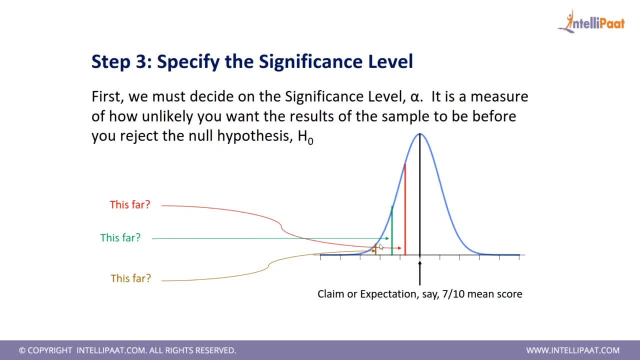 setting the significance level. how sure, how sure you are, I mean 95%, sure you are that a mean which you are looking is lying here or not? so what I am setting here now is the. yet in this third step, I'm specifying the significance level. so what I am telling 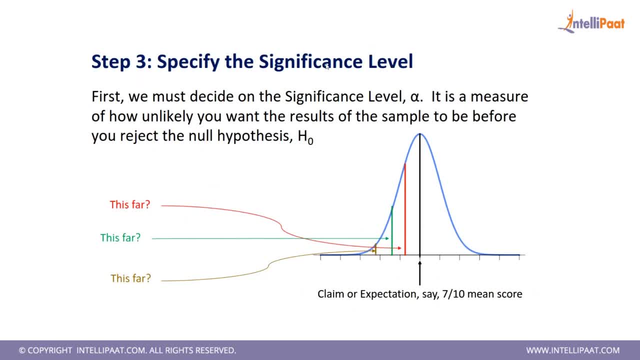 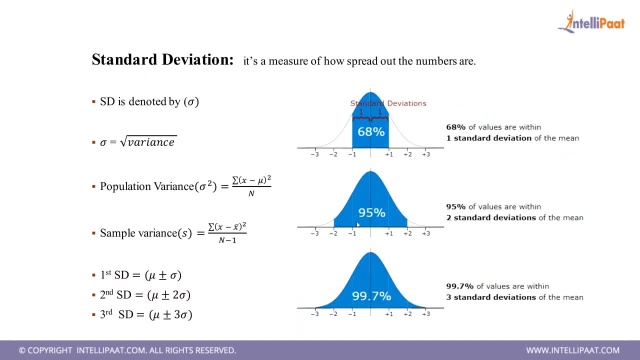 now is the yet that significance level. I'm setting it either to follow this or to follow this here or not. so what I am setting determines having this shape or exactly what I want, because when I don't know, i'm setting it either to follow this or to follow this, or to follow this. so 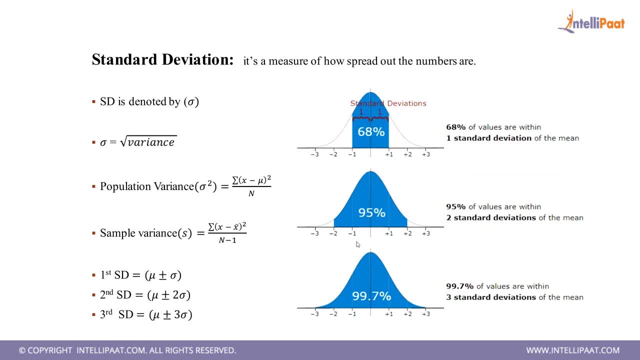 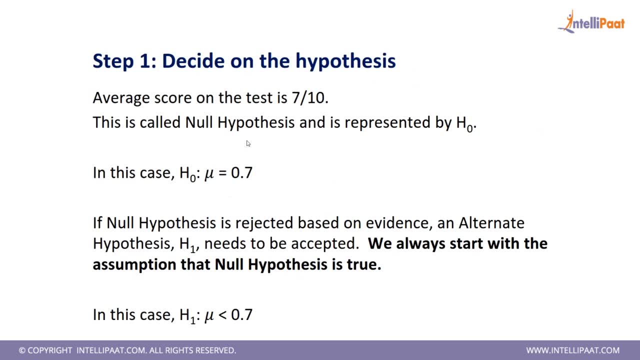 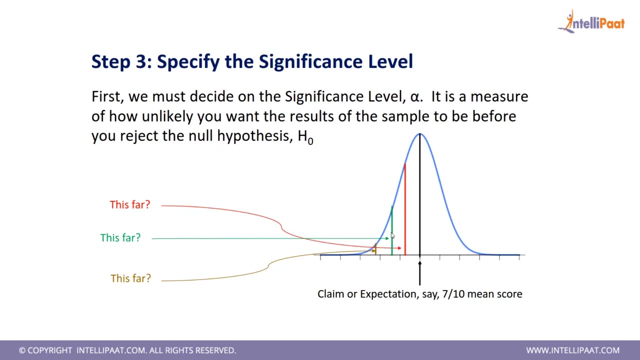 generally we 95%, we will consider. Let's say, I'm considering the significance levels at 95%. so at this point I am deciding that how far it should be, it should be like: significance level should be either third standard division, second or this one. so i'm placing it to be like this far, let's say. if it is coming below this, i'll reject, i'll reject. 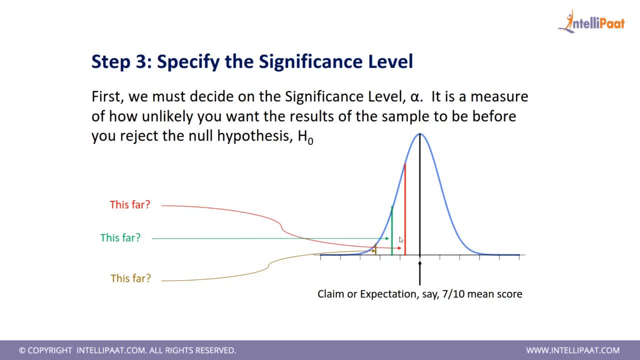 the null hypothesis and, um, the claim made by principle cannot be accepted. that is where, for that, i am uh, giving the significance level, saying that in second standard division i have 95 of the data and the claim. if it is not lying in this value, right, and if the claim is not lying in this, 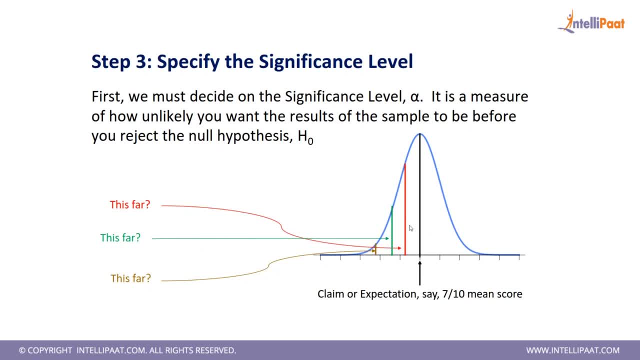 value. i can say that the claim whatever you made, 95. i have lot of data which is like 95 of data, but the data which you are saying is not supporting, then i can reject the hypothesis. so for that i'm setting the significance. two: standard deviation is 95, right, so i'm setting that actually. 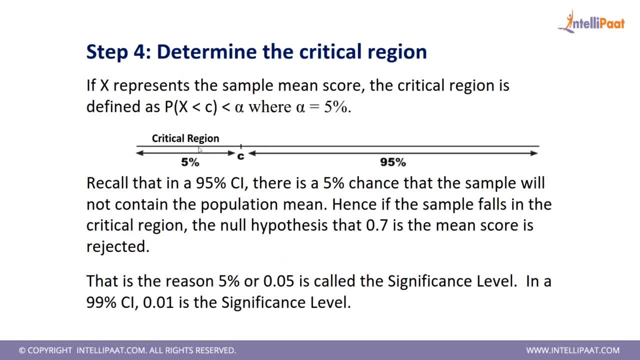 if you see here, you reject the claim, what is being made, and accept the alternate saying that your school doesn't uh have average of seven bands, or something like that. that is where you decide, based on the critical region, so to set what sort of- uh confident interval range. i was doing this. 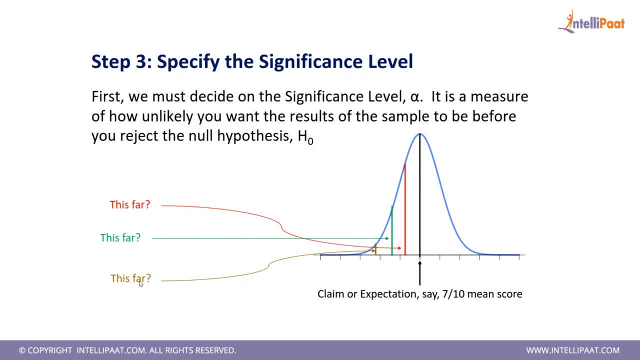 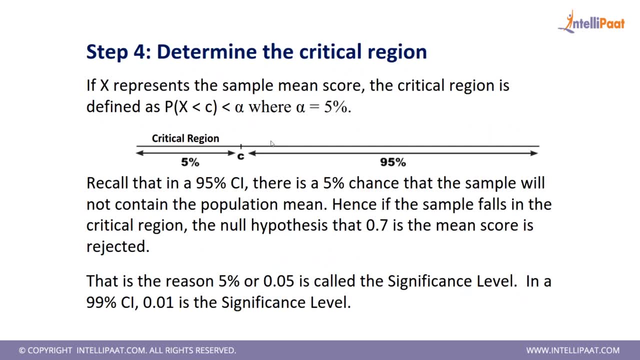 this far, this far or this far. you can go either 95 or either 68 or generally people go with large, of large data, which is 95. if that value, whatever z score value, comes in in this range, right then whatever claim has been made is good enough. if that value doesn't come in the the mean value, 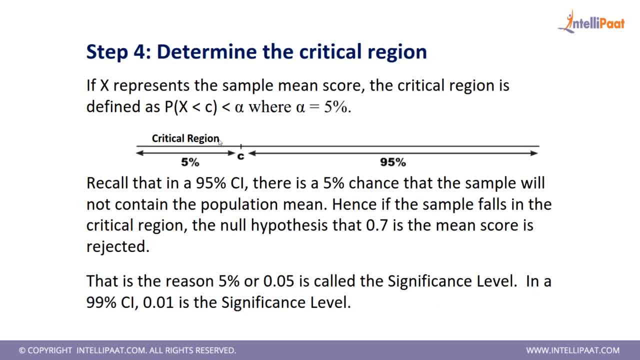 or the standard deviation. uh, the z score value comes in in the four percent or something like that. that gives you that the claim is not supporting you because only five percent of the data is supporting your claim. right, whatever claim you made, the z score gives you saying that five percent of the data is supporting you all. 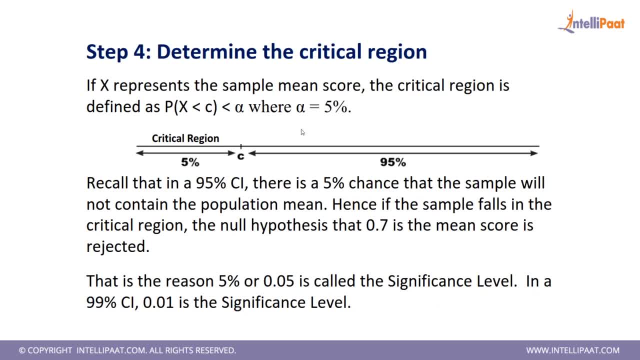 other 95 percent of the data is not supporting your claim. that is where you accept or reject is. give you the critical regions idea. so when it comes above the critical region, you are saying that 95 percent of the data, which is raw data, is supporting your claim. that's all. 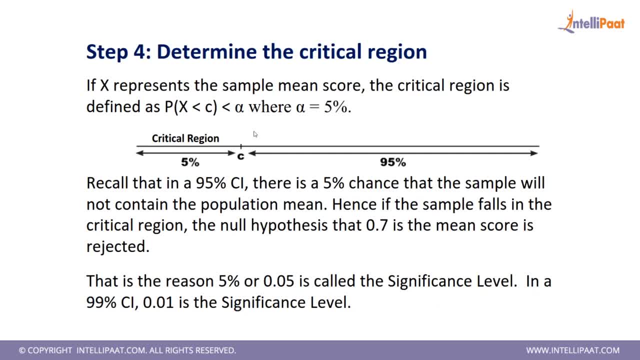 okay, recall that, like 95 percent of critical region, there is five percent. the sample will not contain the population mean. that is where, uh, what i want to pull it out, saying that five percent of the region, it will not have exactly your mean line, right, the entire mean and only five percent of. 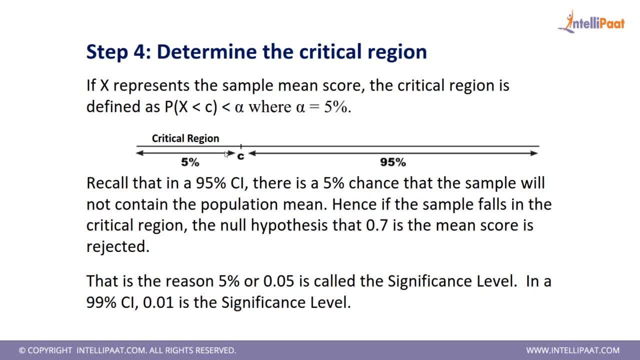 the data is supporting your claim. that is where you accept or reject that and say: if the sample falls below that level, that means that the sample is not supporting your claim. that is where you accept or reject that. hence, if the sample falls below that level, then you are not going to be able to. 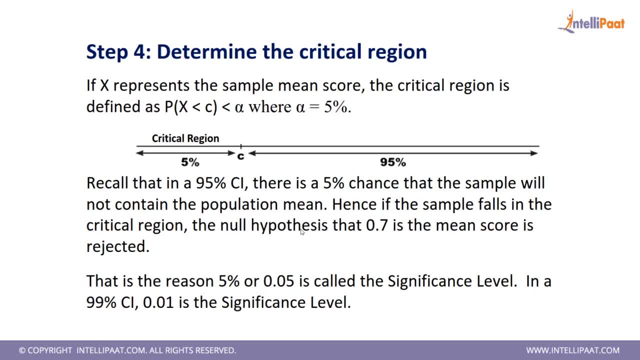 support your claim. if the sample falls in the critical region, the null hypothesis, that is 0.7. the null hypothesis will be rejected if it is lying in the critical region, right? so significance level is the one which you set for, either 95 percent in 99 critical region. uh, confidence interval. confidence interval is. gives you that. 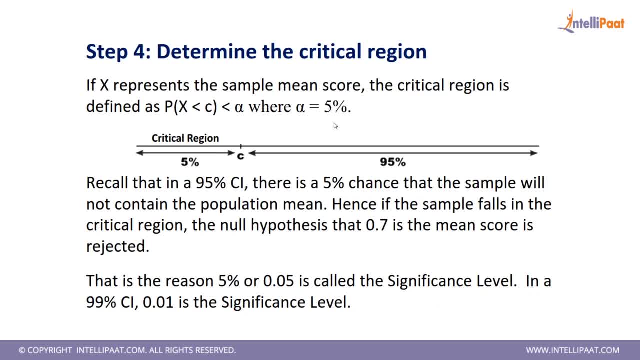 how, how much data you want the claim to be supported. so in our case, what we are doing is we are saying that whenever we get a support of 95 percent data support for the claim made, if we are getting 95 percent of the support from the data, then we are saying that it can be accepted. 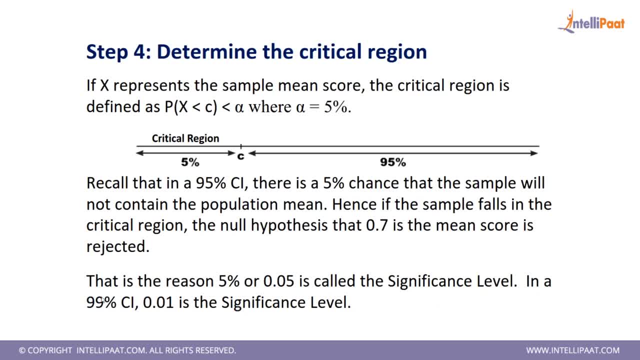 some cases we need a strong uh significance level, saying that you should get a support of 99 percent, then only your uh value can be accepted or rejected on that. so that point of time your critical region would be one percent. so here, if you get a support of 99 percent, then only your claim can be accepted. otherwise, 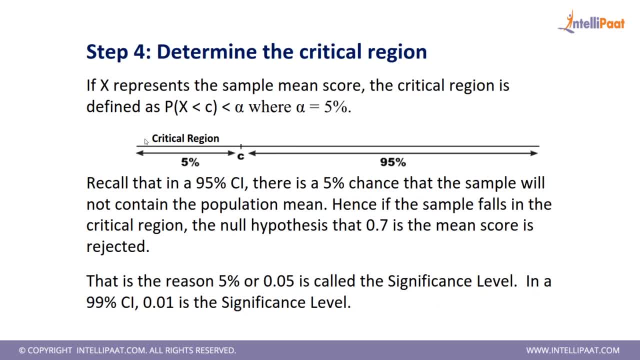 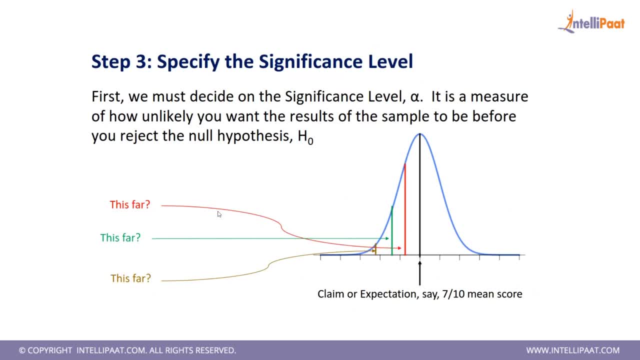 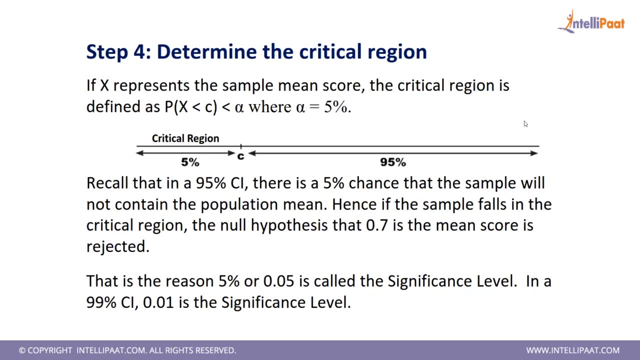 your claim can be rejected because it is there in the critical region. right, that is way what we were doing in this earlier slides. you are setting the support or confidence, uh significance level, how significant the data should support, how much data should support for your claim. okay, and sometimes problem only says that you. you should test this using 95 percent, uh, 90 percent, 95. 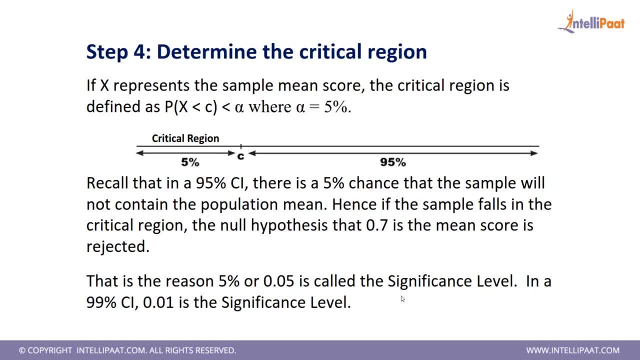 percent claims. right, if they will only define. if 90 of the data is supporting your claim, then you can uh conclude that null hypothesis can be accepted. if it is not like 95 or 90 data is not supporting your claim, you can reject that. okay, the problem statement would be given in in such cases: uh, they will only define that. 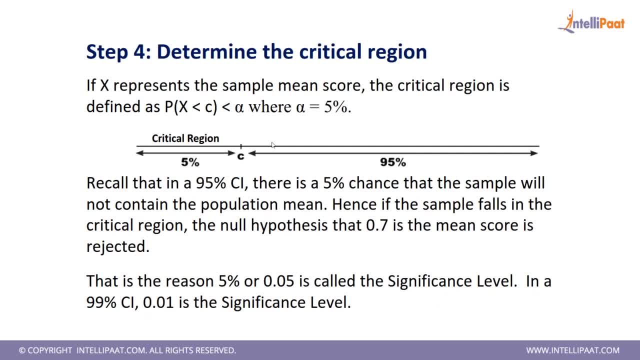 starting from this, it has fallen in 17 percent, not in within five percent, right? so if you see the score, you got 17 percent, which is more than the five percent value. so it is there in the this region. so your claim will be 75 percent of the data. 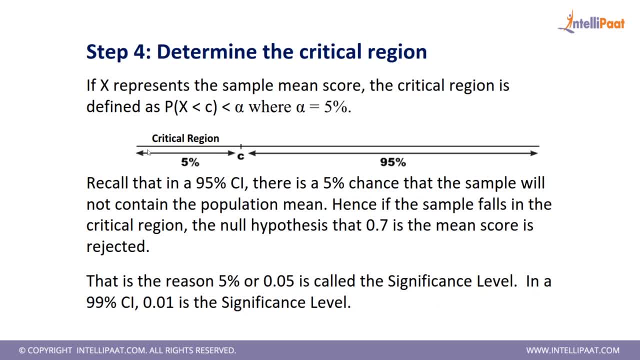 yes, of supporting saying that when you took a sample of class of 40 students, are probably whatever 40 students in the entire stuff, whatever the claim has been made and that value fallen into the 95 data support right. your claim is in this region, your null. 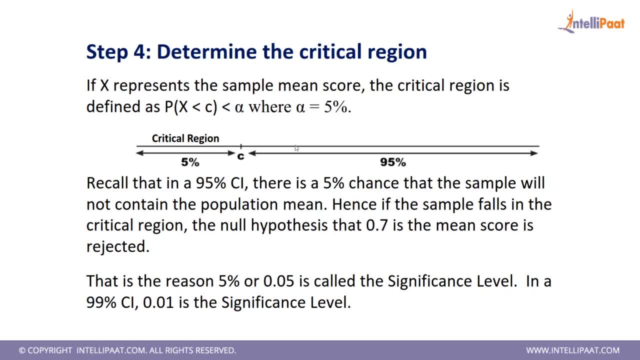 hypothesis will be accepted. that is where we will. we will look that first. understand the critical region and the significance level. it is 99% critical confidence interval. your significance critical region is one person. whenever it is 95%, your critical region would be 5% whenever it is 90%. 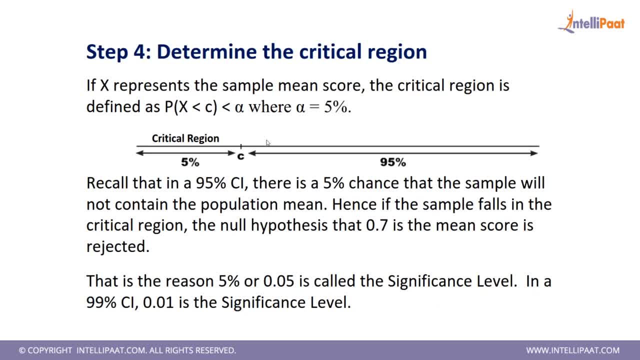 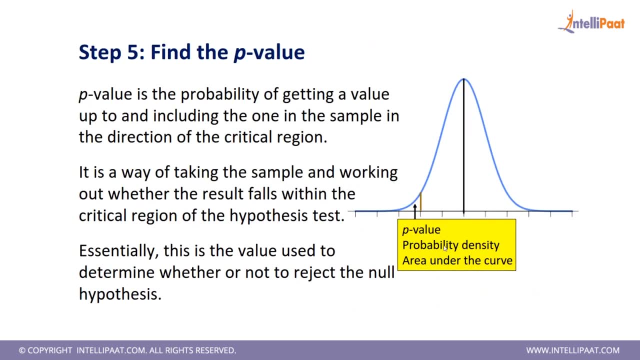 your critical region would be 10%. okay, so determine the critical region is one step. just hundred minus. whatever the confidence interval you are looking for, those things are there. so the probability value: if it is lying under the critical region, you will reject the null hypothesis. reject the null. 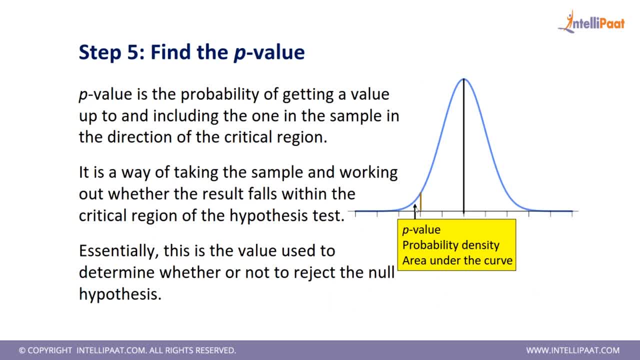 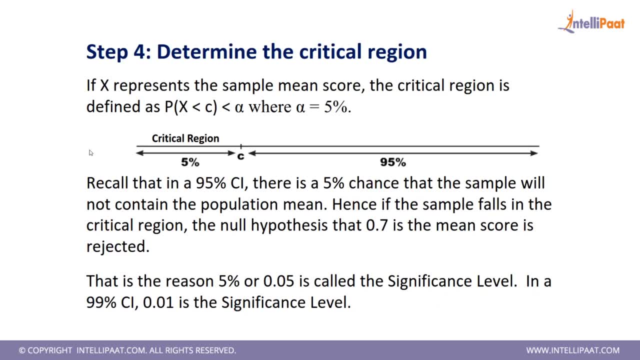 hypothesis when the value is falling in critical region. let's say, your value is falling in critical region, saying that only 5% of the data, entire data, is supporting your claim. right, so this is critical. will not be accepted: only 5% people are supporting your claim. 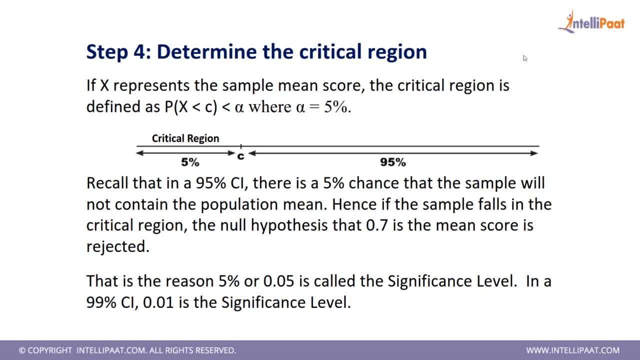 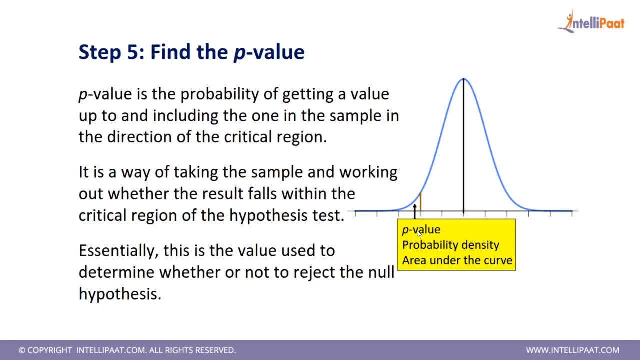 not the 95%. so that is where the probability value tells you. so now those Z score is important, right? Z score is important instead of like standard deviation value and all those things Z score is in. this gives you the significance the p-value in provide p-value is the probability of getting a. 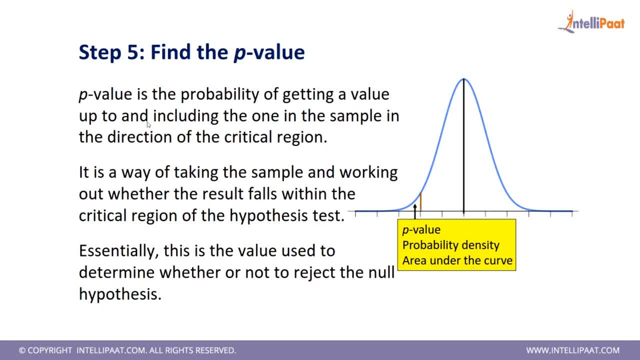 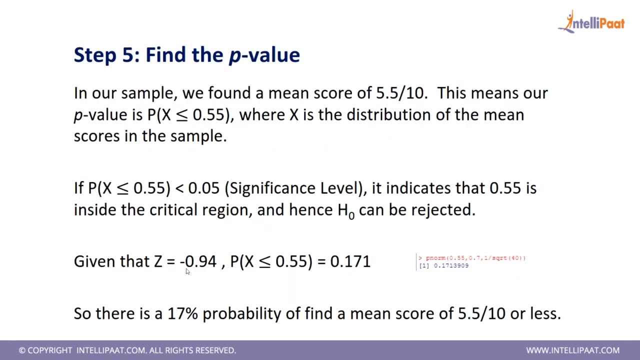 value up to and include the one in the sample in the direction of critical. it gives you the probability actually for a given point, you how far away, and all those things. it gives you the probability. right now. what we're doing is: so we did, we did that. whatever we got it we're setting. it just talks about like if 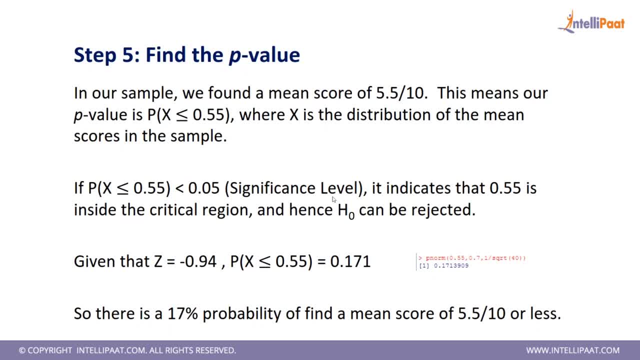 it is falling under. this indicates that can be rejected or not, and all those things. that is defining, so that we got the value to be this one, 17.1. so there is probability of finding mean score or lesser. so whatever is there, it is. it is there in the in the good region. 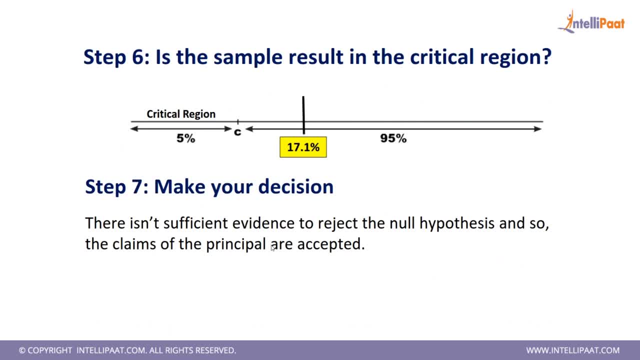 so what we'll do. so there is, there isn't sufficient evidence to reject the null hypothesis, so the claim of the principle can be accepted. right, your claim can is supported by 95 percent of the data. that is where you are. you are looking for. got it any doubts now? so first, find the z-score, set your critical region. how much support? 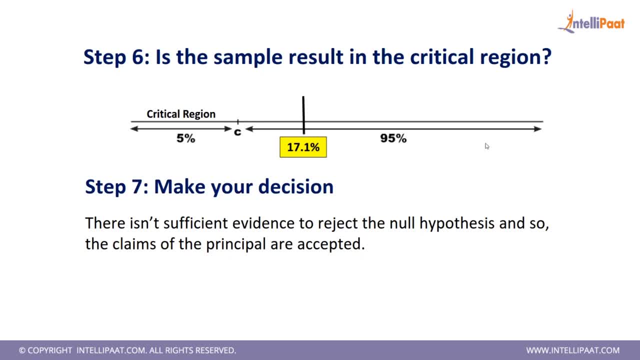 you need for the evidence or how much support you need that you define that. you define that using alpha value, the significance value. so based on that, based on that, you will decide why, whether to accept it or reject it. let's say in the in the example- I'm putting another example there- whether 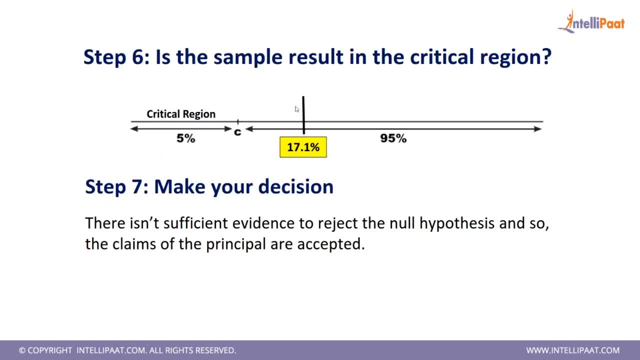 to reject, or one flavor is accepting, one flavor is rejecting. I'm showing there. so what happens is if you say that critical of the value which came out to be one 17- right, it would have been come as four percent- you would have rejected the null hypothesis, saying that your claim. 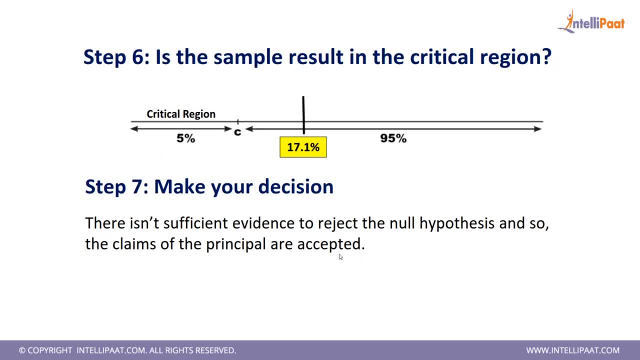 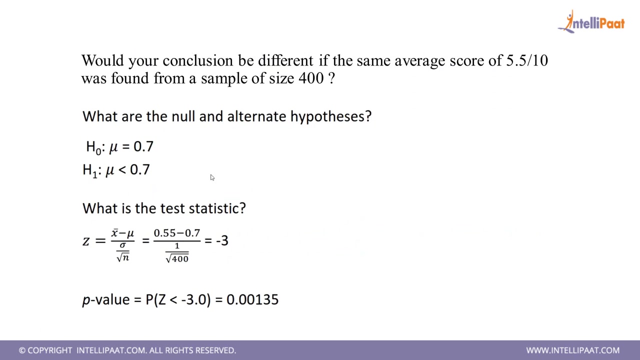 of the principle is not acceptable is what you can conclude if this value turned had turned out to be like four percent. is this intuition? is whatever z-score you got that 95 percent support you are getting, or five percent support everybody. you average score had been with a sample of 400, it was earlier 40, uh, 40 students were involved in. 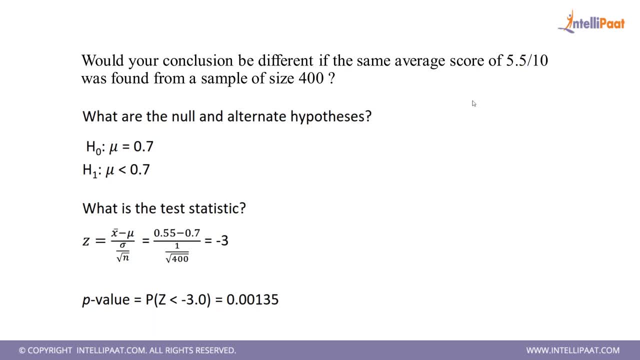 that and the mean turned out to be uh 5.5. now the number of student has increased so the mean would drastically shift right. so earlier the mean was somewhere around in the in this normal uh 95. now we will check what actually it is. so when i passed in the values, 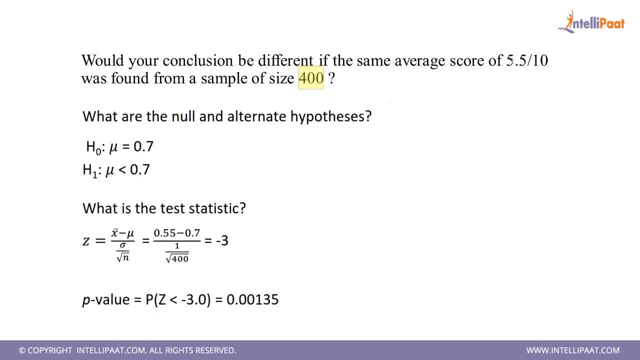 here, right. x value what? whatever we have divided by 10, right, this one, 0.55, is your. that the value, the mean value of the population, is 0.7, which is based on the claim and the standard division is one. the number of elements involved in it is 400. it gives you minus three. so for that. 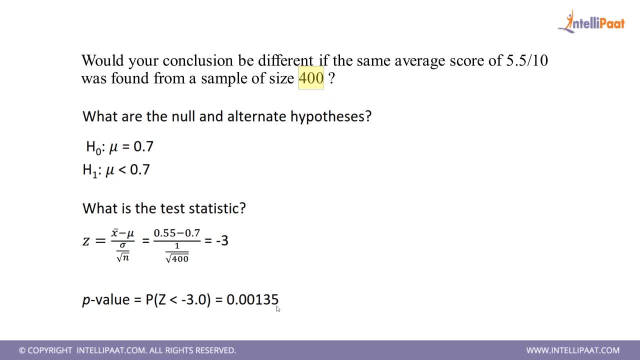 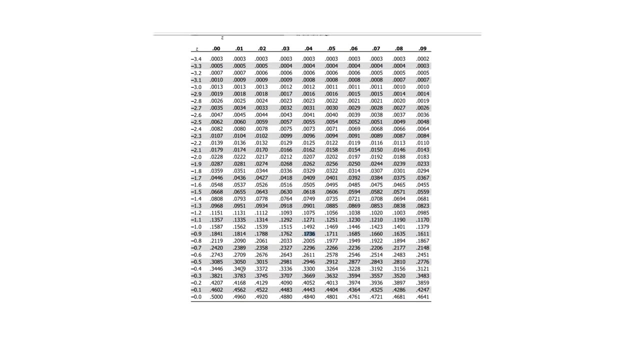 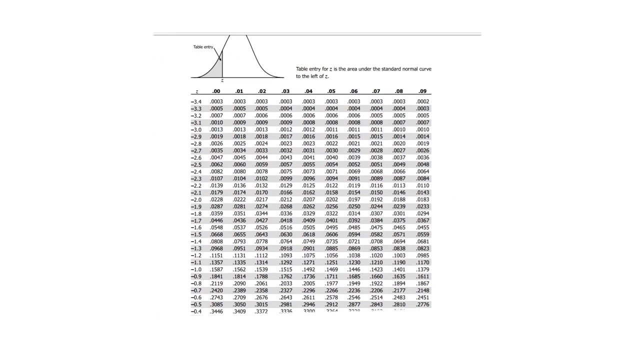 probability value will be somewhere around zero, zero, one, three. so zero point, zero, zero, one like point. one percent is your value, if you just see minus three value rate. right, this is the value. okay, this is the value we. we will be getting exactly this: one, one, three, five. now what you do, since the value is lesser than the significance level of 0.05. 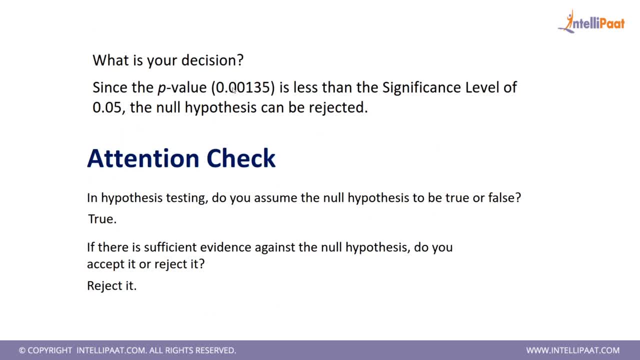 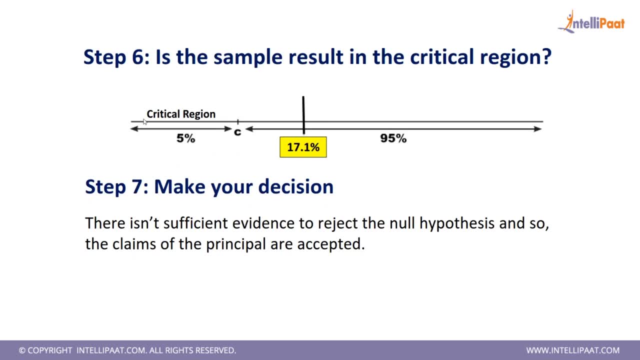 like five percent. it is closer to point one percent. so null hypothesis can be rejected. if you consider this, it is coming somewhere here. you reject the null hypothesis, two flavors of it. when is when we are accepting, then we are rejecting that. okay, this is how you do hypothesis testing based on statistical evidence. whatever claim has been what we were. 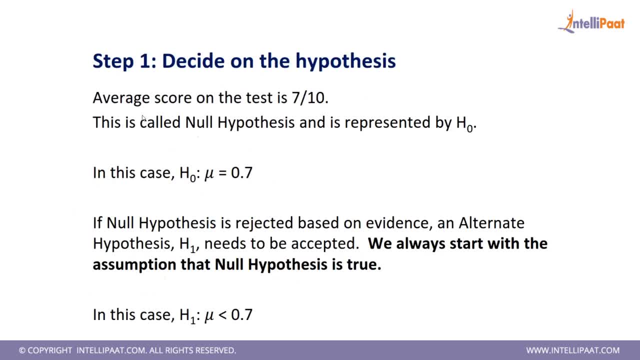 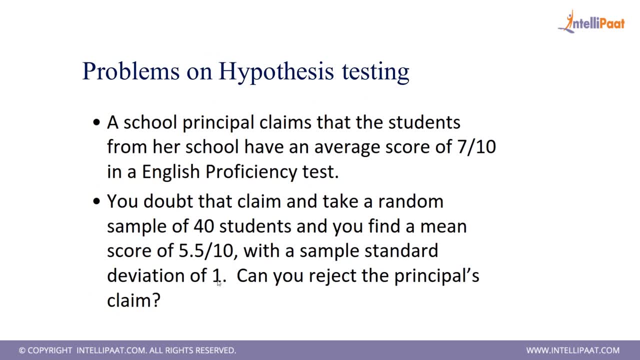 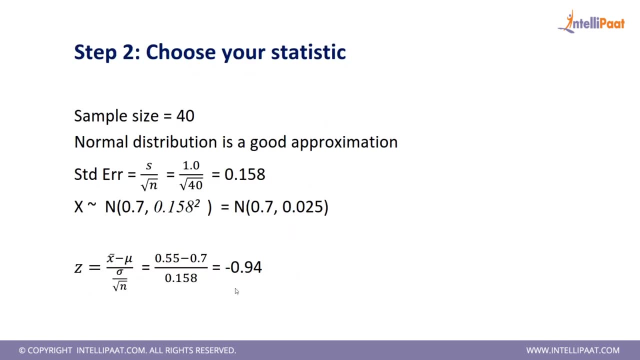 doing what whatever claim has been made by principle. we did a statistical study saying that we took the sample of the student, mean of those, whatever we got, and standard deviation to that of number of student involved. we we generated some z score value for it. we took the. once we got the z score, we evaluated the probability for that. 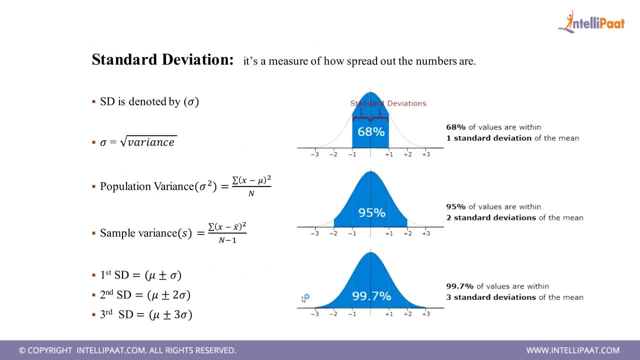 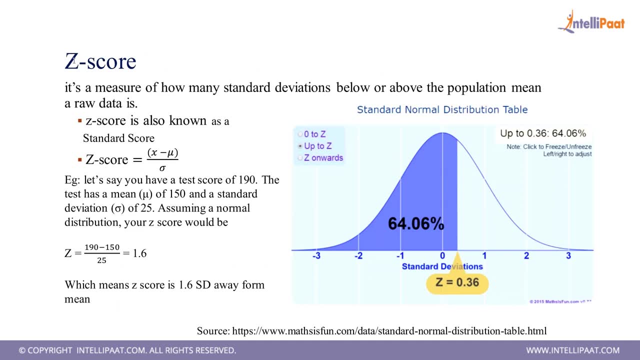 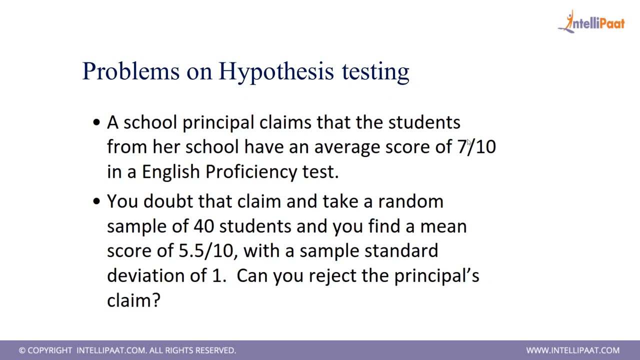 to understand this, where it lies. how much percentage in range? uh, it lies. that is where the importance of z score and its probability. so principle is claiming that average students would get at an average, they, each student, would score seven bands out of ten. but when i do a real survey, 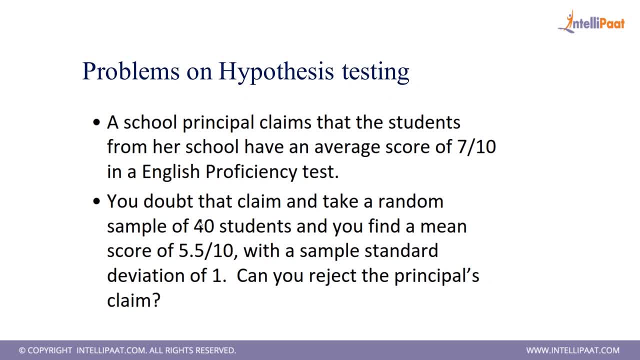 of a class i found that out of 40 students mean was not exactly seven, it was 5.5. right, when i did a class survey out of, let's say this was for thousand students for the entire school, principal was saying that they used to get a mean average. a score in english proficiency test was seven. 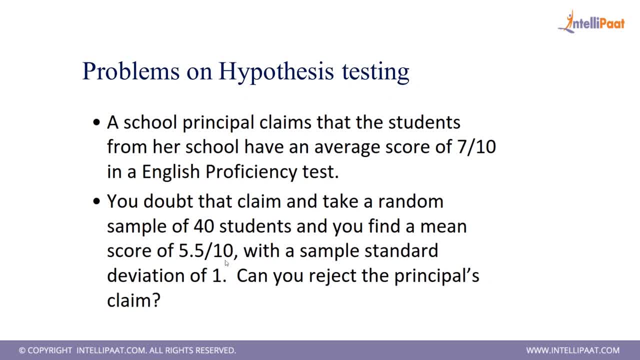 but when i actually drill down i could have done for the entire population, but since some cases we need not to go to the entire population, get those all data. we drill down to one particular class and see if one class is doing well, um, supporting this or not. so when i go to the uh sample, we did a. 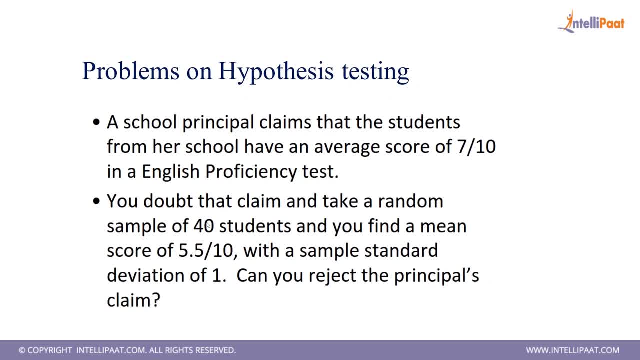 random sample right when of 40 students- either it can be a class or from various classes- some 40s to elements, i mean students- have been picked in this analysis: 40 students and their score- when i mean those, i got a score to be 5.5, which is not supporting principles claim i could have. 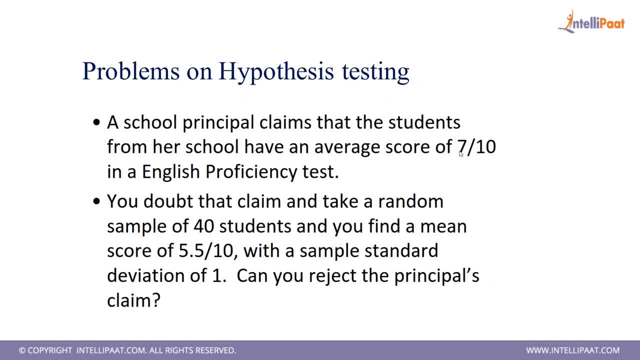 directly said that this is not good. whatever claim you're doing is not good. but unless you do the statistical evidence right, then till that point you cannot deny this uh, this, uh claim. that is what hypothesis test gives you. that is what the intuition behind. so what is actually hypothesis testing? 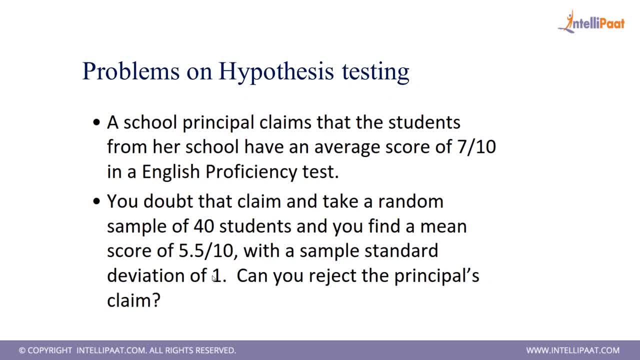 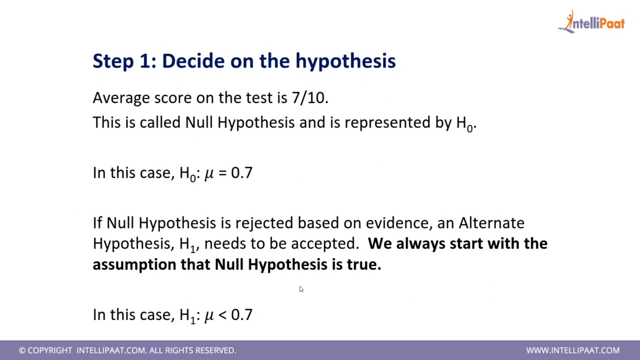 hypothesis is nothing but the claims or a statement. so it's a random sample. it can be any class it can, if you try out with various sample saying 40 student saying uh with different, different uh flavors of it. so main thing is need to whenever uh students are, so it. 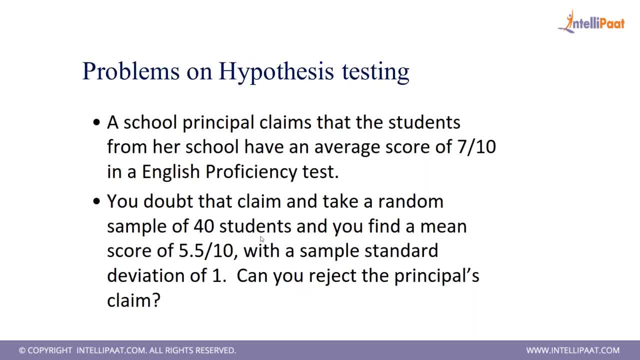 will not be every time. standard division means and all will be given. they'll just give you some 40 students their marks. you try to evaluate mean. what is the mean actually? so you get some mean around like 40 students. the values would be ranging from 1 to 5, 1 to 10. sorry, right. so when i take mean it,